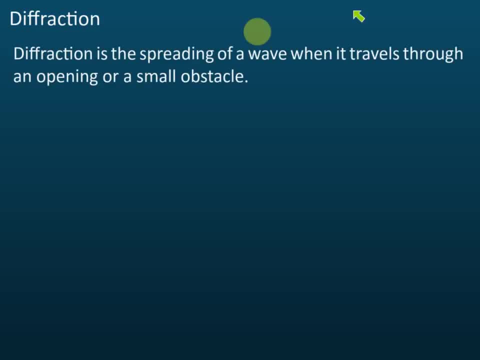 okay, what is diffractions? what is diffractions? diffraction is the spreadings. so this is the most important words here is the spreadings. okay, so diffraction is the spreadings of the wave when it travels through an openings or small obstacles, passes through an openings or passes through the 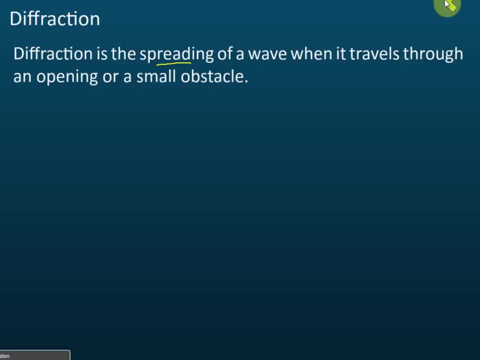 site of a small obstacles. so, uh, that is the definition for diffractions and you need to memorize. you must memorize this, um, okay, because in exam they will ask you: what is the fraction? what is mean by diffractions? are then, this is what you need to give. okay, examples, uh, 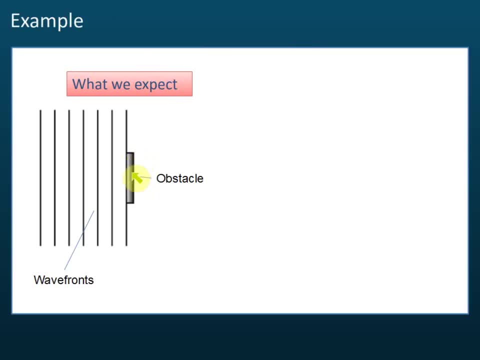 let's say we have a small obstacle here. okay, and this is a wave and the wave, actually the wave move from left to right. for this one, huh, the wave moved from left to right. okay, when the wave move from left to right. okay, when the wave move from left to right. okay, when the wave. 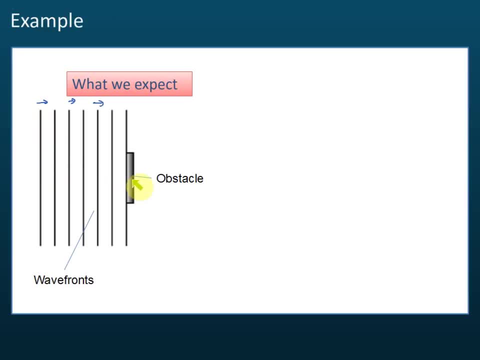 move and it hit the obstacles. it hit the obstacles, it will be reflected back. hit obstacle, reflected back. this one, no problems. okay, we have learned reflections of wave. okay, but then what will happen to the wave at this two, at the two side? what will happen to this, the wave here? 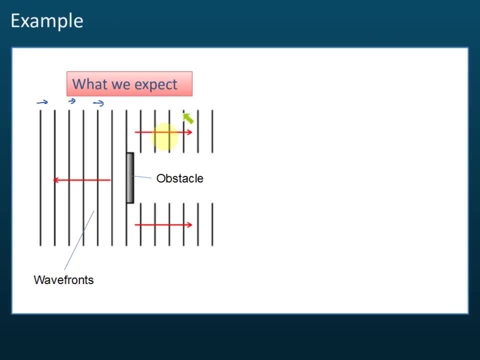 okay, we expect that this wave, it will move forwards like this. right, okay, this one, it hit the obstacle, it will bounce back, reflect back, but for those wave which doesn't hit the obstacles, so it can move forwards like this. so this is what we expect, okay, what we expect, but the reality is. 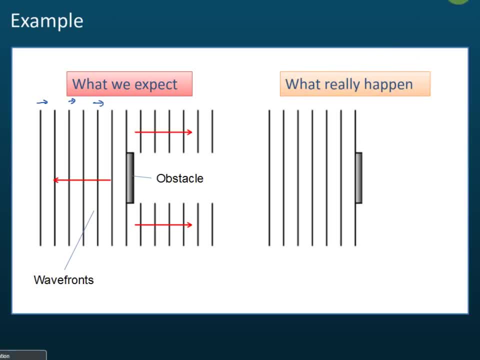 what happened is okay. what really happened is this one: it hit the obstacle, bounce back, no problems, okay. but for the wave here: okay, it does not move forwards like this. but after passes through the obstacle is spread, okay. okay, you see, yeah, this one is it move forwards in a straight line, but this one after it passes.